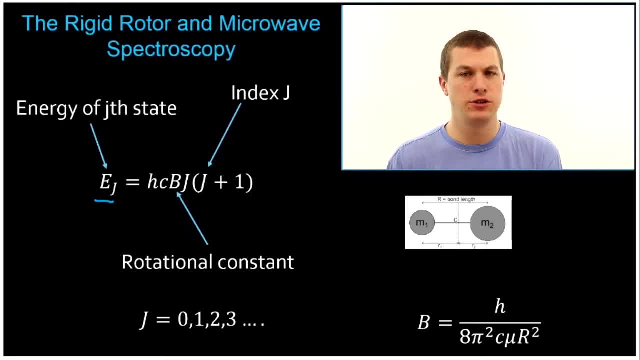 your particle. in the box, We have the energy of the j-th state. In this case, we use j instead of n, but the idea is the same. We're just labeling every single successive energy level and we use j In this case. j can run from 0,, 1,, 2,, 3 up to infinity, And you'll notice that the energy 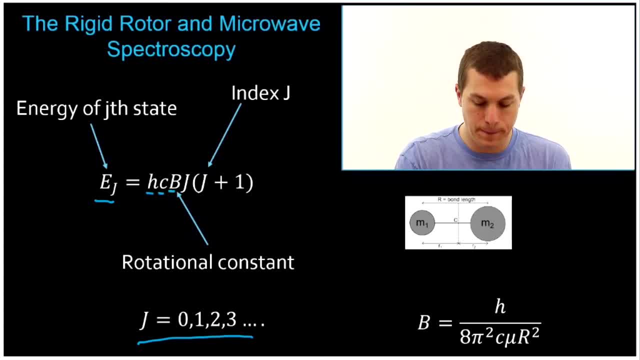 depends on Planck's constant, the speed of light, and this b, which is called the rotational constant, And we'll talk more about the rotational constant in a minute. For now, let's look at how j affects our energy levels. Well, we have j appearing once, twice, and one of 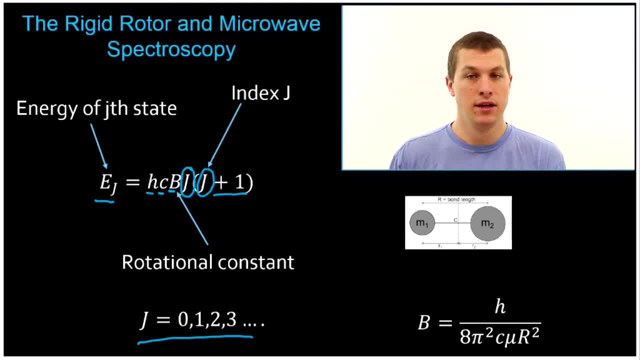 the times it appears, we add one to it and then we multiply it by j, And so this is going to be a little bit like our particle in the box- particle in the box where our energy levels are going to get farther and farther and farther apart. 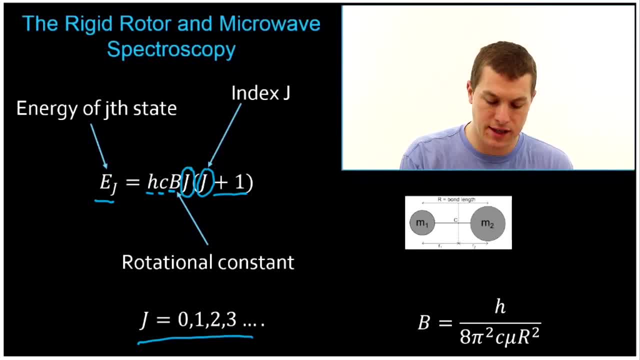 as we go higher in j, But it's a little different than our particle in the box in that we add one to that first instance of j. Let's take a look at what that actually does to our energy spacings because, remember, it's the transition between our energy spacing levels that will tell us about what. 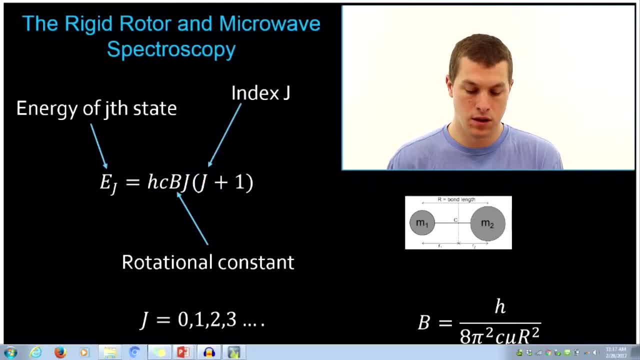 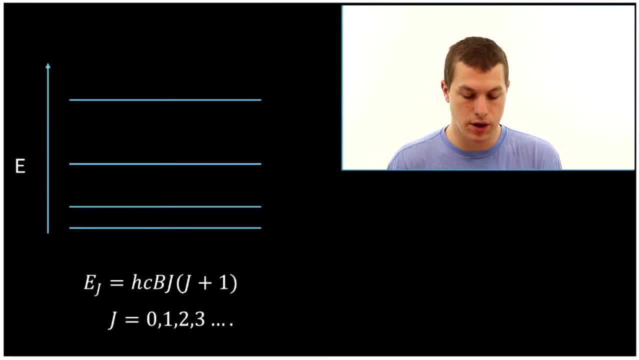 wavelengths of radiation will be absorbed. So here I have the different energy levels laid out for our rigid rotor, And remember that we can calculate them by plugging in the appropriate j. So let's think about what happens when we plug in zero. Well, when we plug in zero, that means that 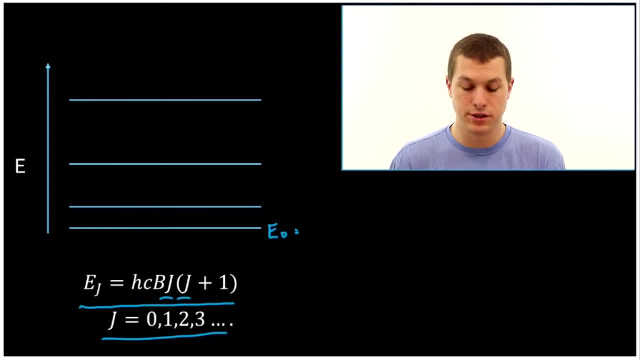 j is zero and that j is zero, And so we're multiplying the whole thing by zero. So the energy of our zero state is actually zero, And that means that in our ground state our molecule is not rotating. So we can have molecules that aren't rotating at all. This is different, you. 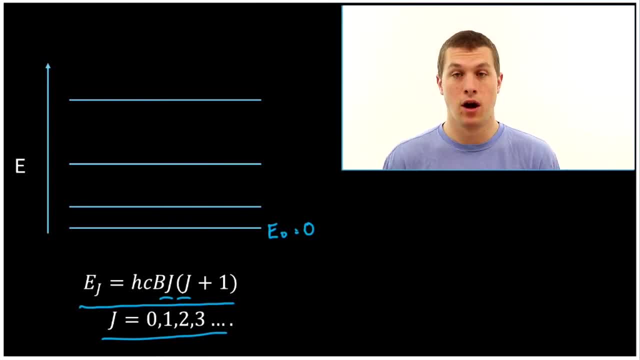 recall, than the harmonic oscillator. The harmonic oscillator in the ground state, our molecules are always vibrating. But for the rigid rotor in the ground state, our molecules can just be still. That is not rotating. Alright. what happens when we plug in j of one? Well, if we 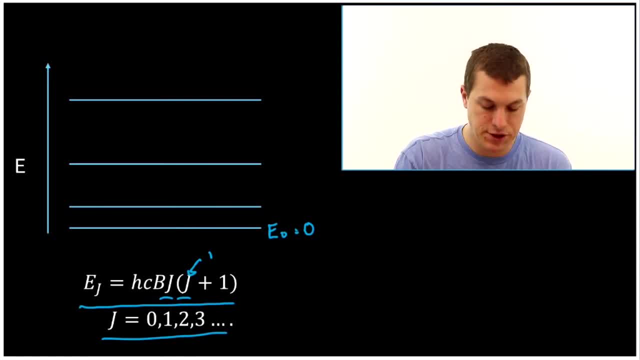 plug in one to this guy, we're going to get hcb times one times one plus one, So that's going to turn out to be two hcb. Okay, let's think about plugging in: j equals two. When I plug in, j equals. 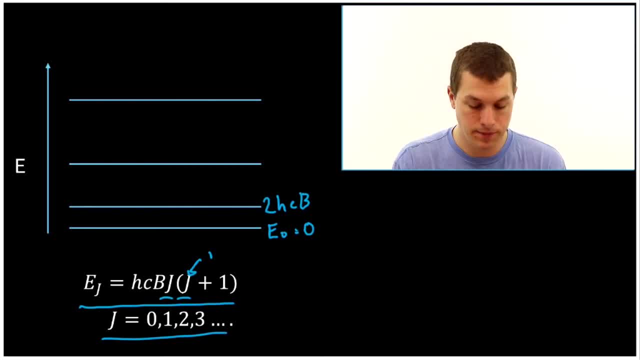 two. I'm going to put in two, add one, that gives me three. And then I'm going to multiply it by two, That's going to give me six hcb. And then let's plug in three. Then I plug in three. I'm going to add one because it says j plus one, So that gives me four. 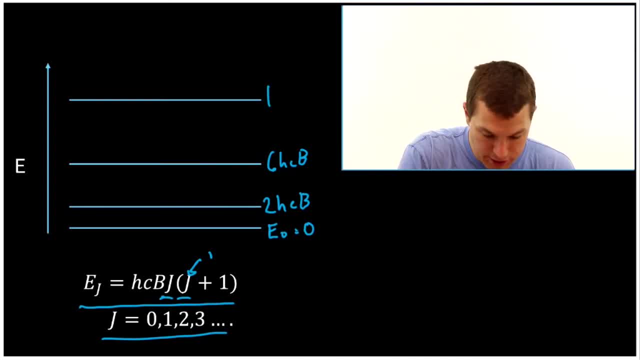 And then I multiply it by my three and that's going to give me 12 hcb. So you can see that as my energy goes up, my gaps get farther and farther apart And it turns out that each successive gap gets two hcb farther apart. So you'll notice, between the zero state and the first state we 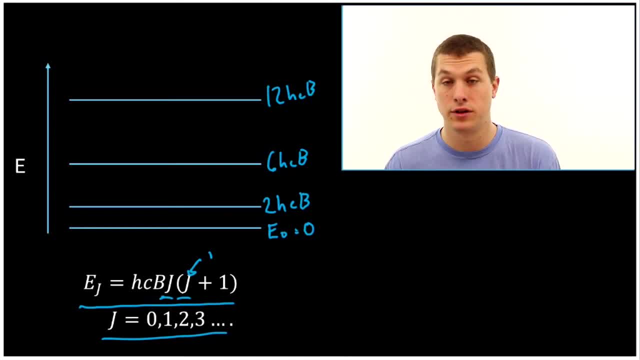 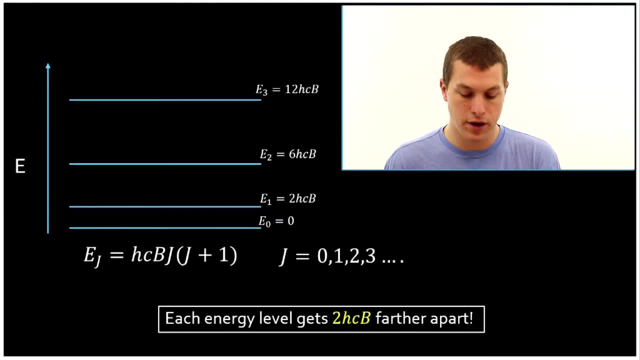 have two hcb And then I plug in three, and then I plug in three, And then I plug in three and then I plug in two hcb. Between the second state and the third state we have four hcb, an additional two hcb. Let's take a look at this written a little more neatly. Here are different energy. 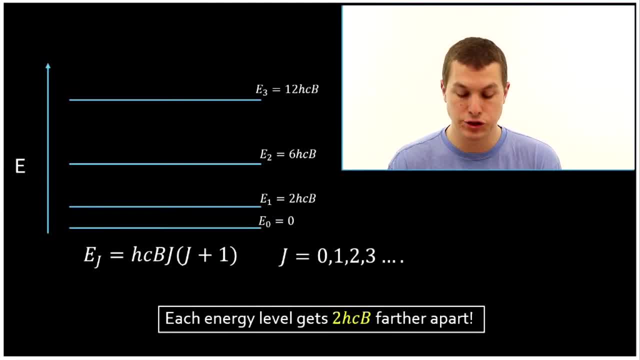 levels, And each time we go up, we get two hcb farther apart, And what that means is, when we look at our microwave spectra, we're going to see a series of peaks, because each of these transitions will be at different energies. Let's take a look at what I mean by that. 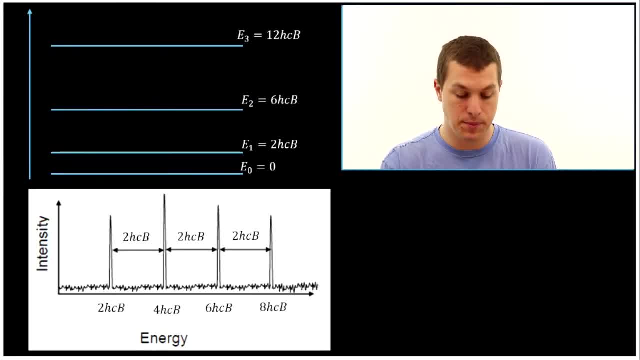 So here you can see that we have two hcb And then I plug in three and then I plug in three. You have in the top are energy levels And in the bottom you have a microwave spectra. This is showing microwave radiation that's been absorbed And you see four peaks: One, two, three, four. 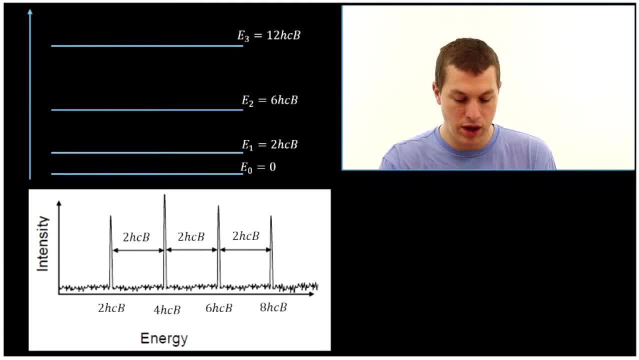 peaks. Let's talk about where each of those peaks comes from. Well, if I put on microwave radiation and my molecule happens to be in the ground state, then what that would do is cause my molecule to transition from e equals zero to e equals one, And that amount of energy would be two hcb. 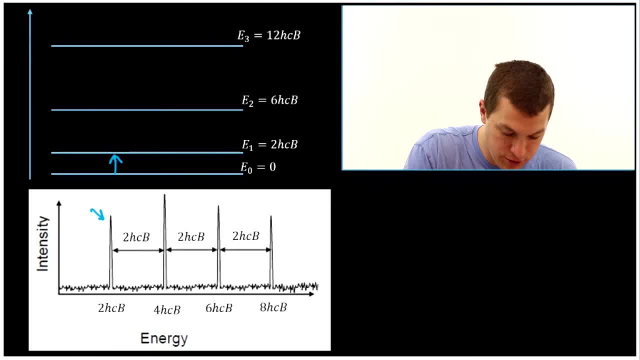 So that's this peak right here. So this turns out to be e zero to e one. On the other hand, if I start out with my molecule in the first excited state and I transition it to the second excited state, that gap is six hcb minus two hcb or four hcb. So that's this guy right here. It turns out to be e. 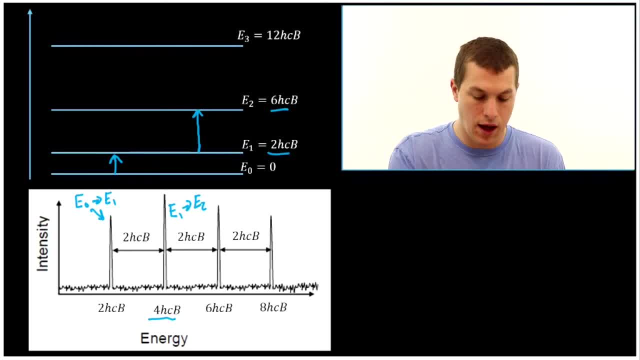 one to e two. On the other hand, it could start in the second state and go to the third state. There I'm going from six hcb to 12 hcb. So that's this peak right here. So that's this peak right here. So 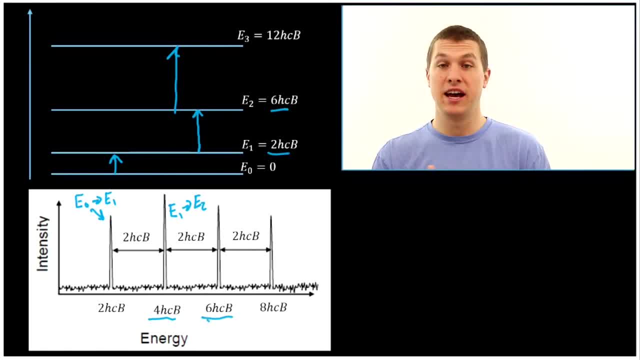 that's six hcb. So that means that I would get out six hcb as the difference. Remember, it's the change in energy that you're seeing show up on the spectra, because what we're doing when we put light on it is we're kicking a molecule from one rotational state up to the next. And if I start, 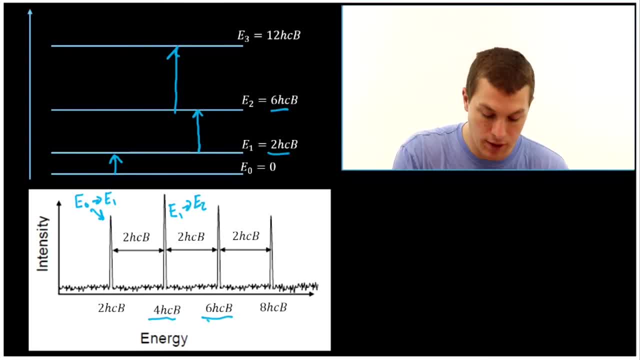 in the second state and go to the third state, my change in energy will be six hcb. So that means this guy is e two to e three And lastly, this peak is e three to e four. So notice that you see four peaks here and that's also different from, say, vibrational spectra. So if I start in the second, 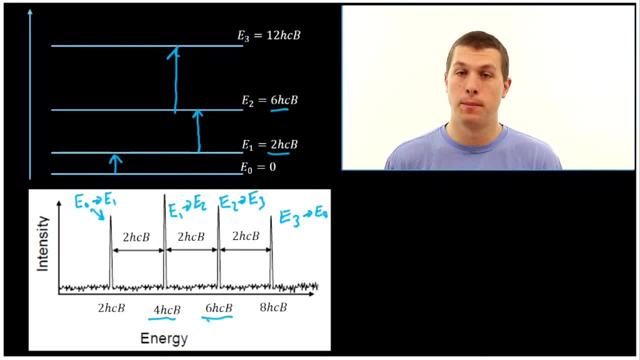 state, you'll see 4 hcb here. So, for example, if I start in the second state, I would see 4 hcb here and the next ones are a lot smaller. So I'm going to do it one by one, one by one, and I'm going to 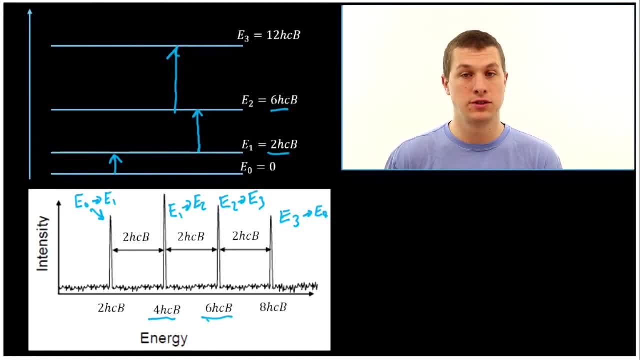 start on the second state, So you'll have moreishing depending on the temperature around that, And then you can start in rcb, where you typically only see one peak. Rotational energies are much lower in energy than vibrational energies, And what that means is that just because of the 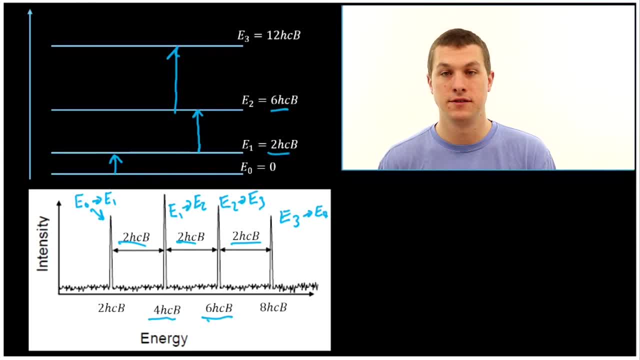 temperature around, we'll have our molecules starting out in different states. So initially, And the reason that is is that every single time we go up in an energy level, we add 2HCB to our spacing. So this is a subtle issue, right. 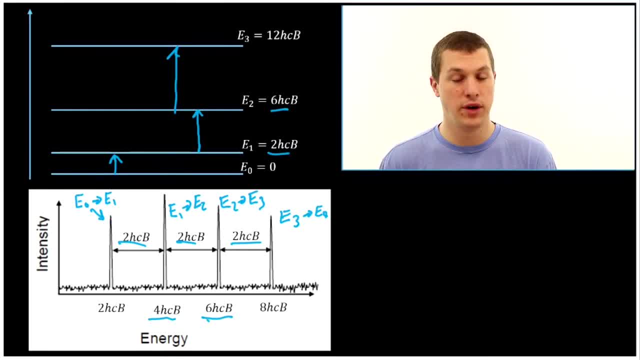 But we go from energy of 0 to 1, and that's 2HCB. We go from energy of 1 to 2, and that's 4HCB. We go from energy of 2 to energy of 3, that's 6HCB. 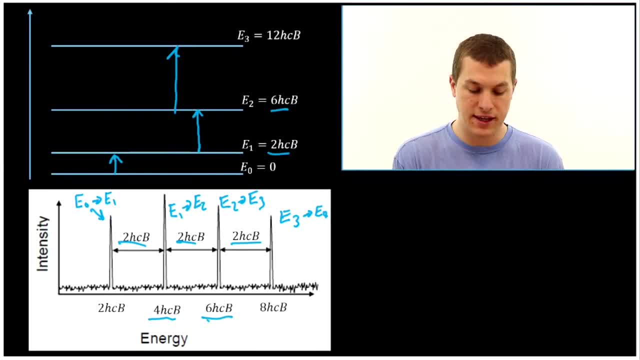 So you notice, each time we're getting 2HCB high there And that means that the gaps between our peaks will always be 2HCB. And that's a really useful fact because when we go and actually measure a spectra, or spectra for the microwave absorption, 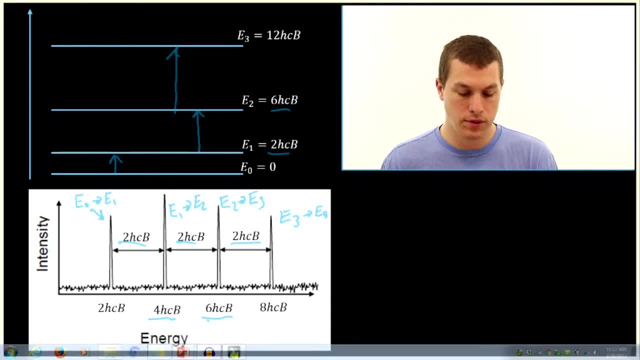 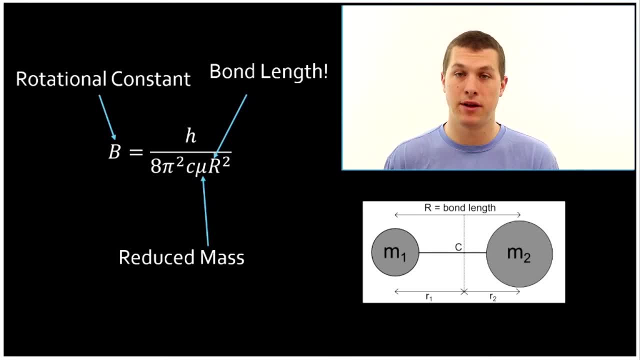 we won't get HCB out, we'll get some energy. So, for example, let's say that we get out 10 EVs. Well, now we can relate that to our microwave constant. Let's talk about that microwave constant and then we'll take a look at the spacing. 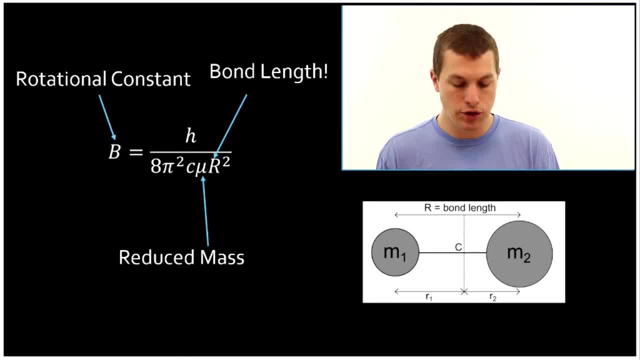 So here's our rotational constant, And you'll notice that if we look at the equation for our rotational constant, we have B, and we have Planck's constant appearing again, and pi and C. But we know what all those things are, so let's focus on the things that we're a little less familiar with. 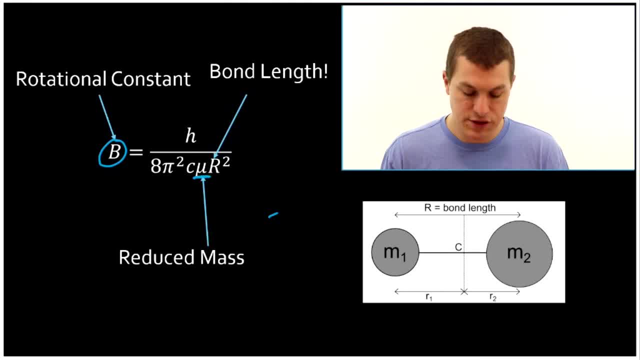 B is the rotational constant. as I've already said, Mu is the reduced mass, And so the reduced mass is just a way to take the fact that we have two masses in our system and combine them into one. It's just basically a math trick. 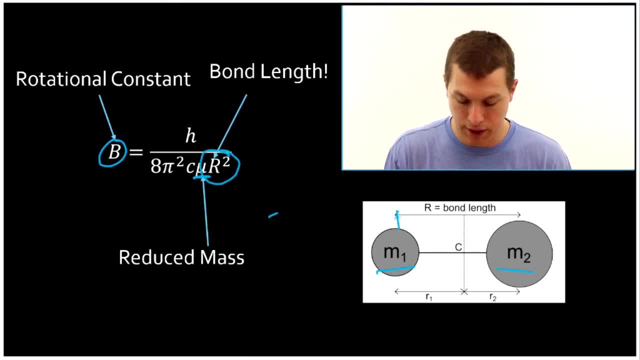 Importantly, we also see this R here, and R is the bond length, And that means that if I have my rotational constant, which I can get from the spacing of my microwave radiation, I can get out bond length, And that's really the key thing that microwave spectroscopy does for us. 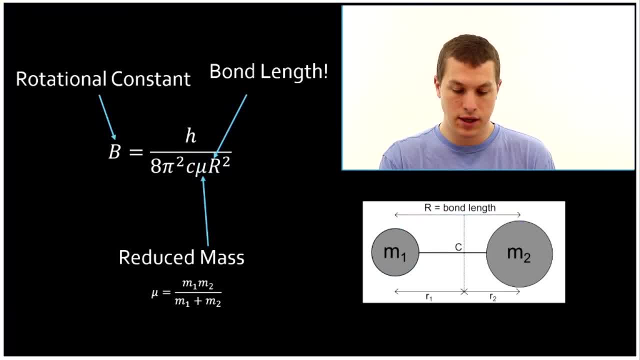 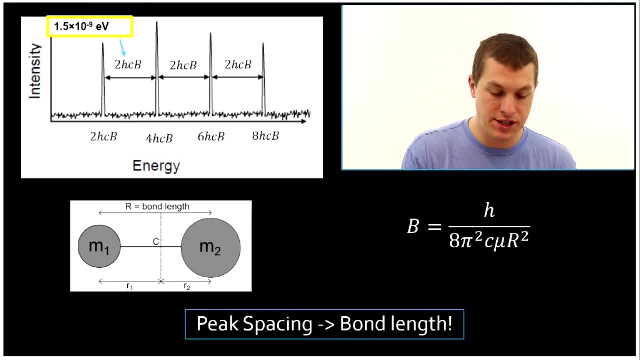 So let's take a look at a specific instance of that. So here what we have is our microwave spectra And if you go into the lab you can measure those gaps. And let's say we measure that it's 1.5 times 10 to the minus 9 EV. 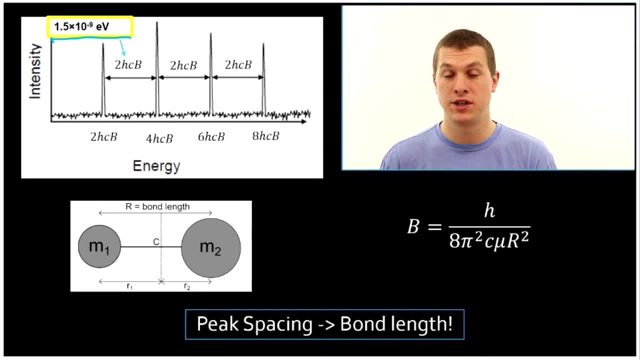 First thing to notice that's a really small amount of energy, And that's because rotational energies are really really small. It's really really easy to kick a molecule from rotating a little bit to rotating a little faster, And that peak spacing, if I know it. 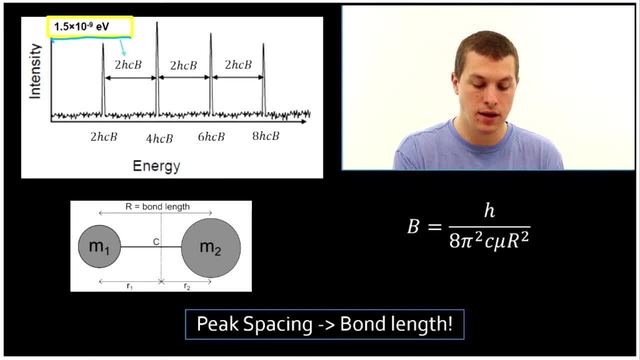 as 1.5 times 10 to the minus 9 EV, and I also know that it's equal to 2HCb. I can calculate the bond length Right Basically from my spectra. I got this equation 1.5 times 10 to the minus 9 EV. 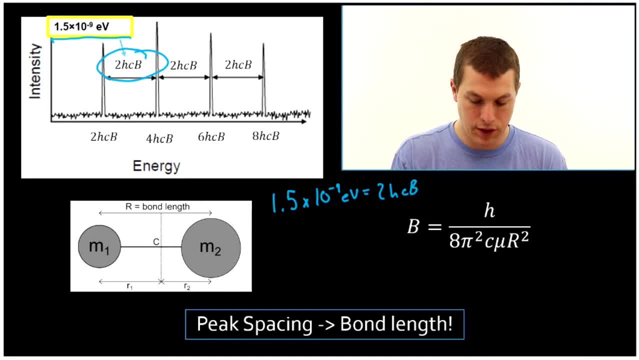 is equal to 2HCb And since I know it's equal to 2HCb, I can calculate the bond length. And since I know it's equal to 2HCb, And since I know it's equal to 2HCb, 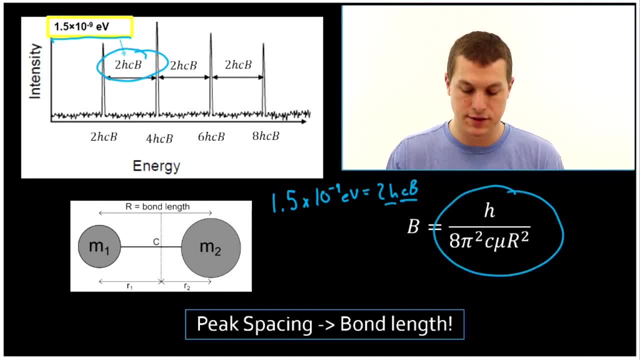 And since I know it's equal to 2HCb h and i know c and i know what my rotational constant is, i can go ahead and get out bond. and that's what microwave spectroscopy does for us. primarily, it allows us to use a rigid 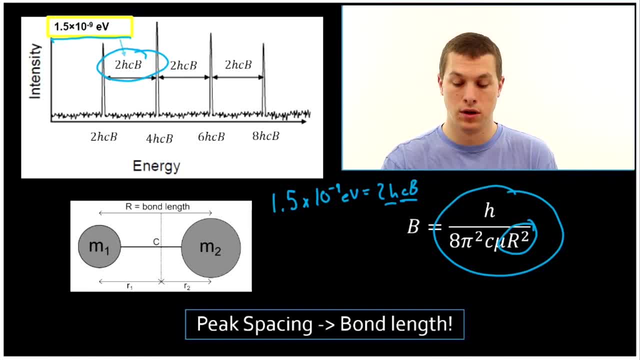 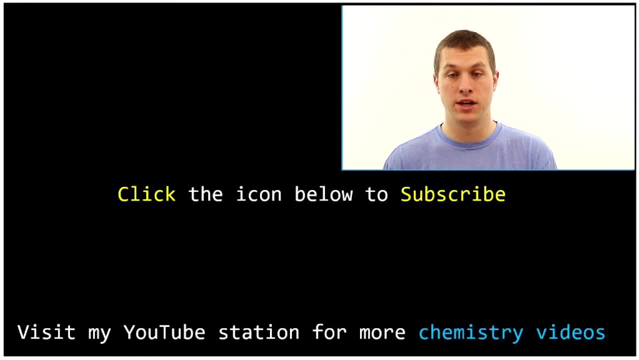 rotor model to figure out the bond length for a diatomic molecule. so in the next video, which i'll link to below, we'll actually go through an example where we calculate the bond length from the rotational constant. thanks for watching this episode of real chemistry. check out the next one to see a practice problem.